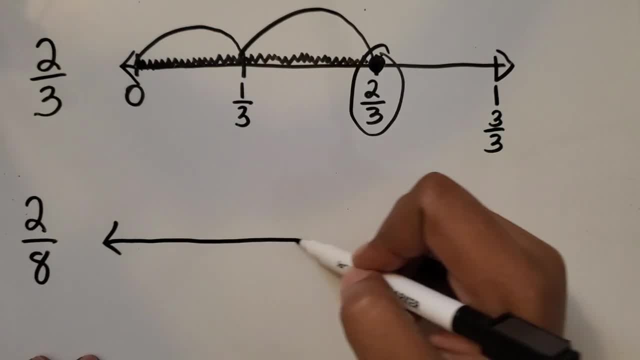 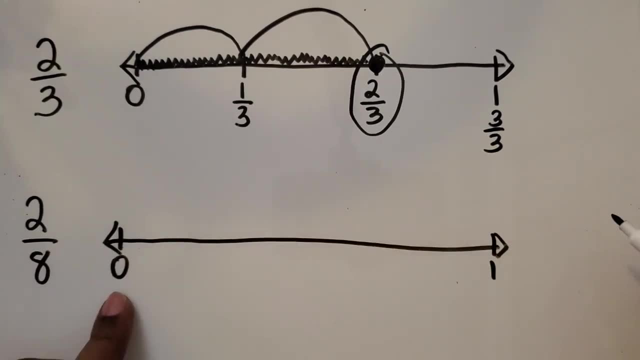 cell in this problem. I'm going to count by saying 1 to 8, 2しくleri, So I'm going to draw same size hole, still representing one hole. So we're going from a distance of zero to one hole. 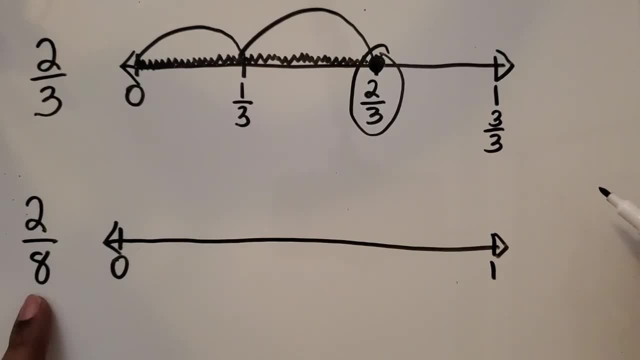 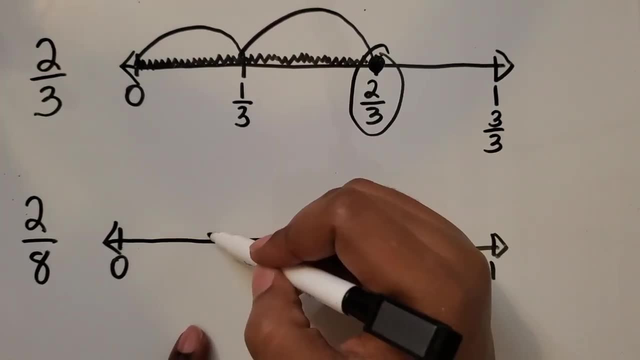 Now I want to partition my number line into eight equal parts. So I'm going to start by partitioning it in half And then for each half I'm going to partition those in half to make fourths, because we have four equal parts. 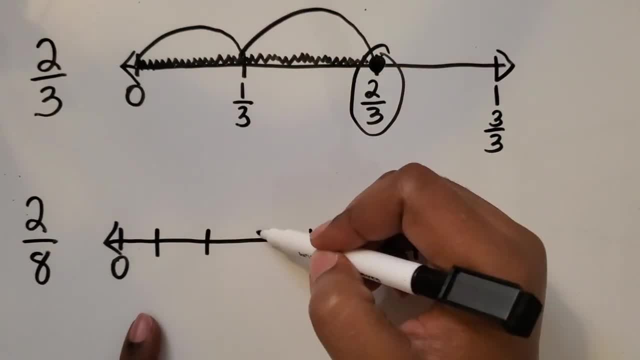 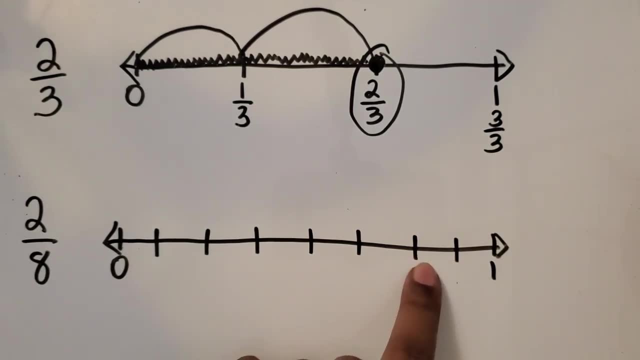 And then for each fourth I'm going to partition each fourth into in half. So now we have eight equal parts. So where is two eighths? So if I start at zero, from zero to the next tick mark, is one out of the eight. 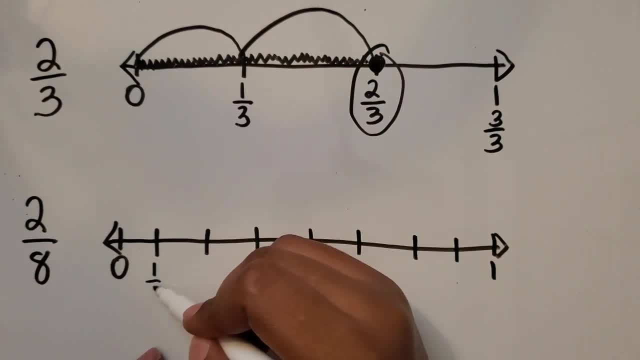 And from that first one let's label it one eighth. From here to here we can do our jumps again. That will be two, Two eighths. Okay, So you can label the rest of your number line or you can leave it like this to show that you found where two eighths is on the number line. 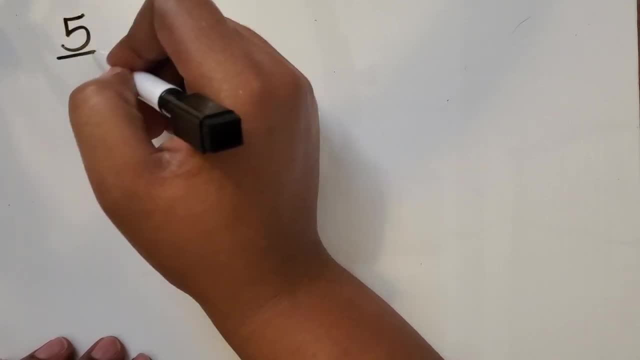 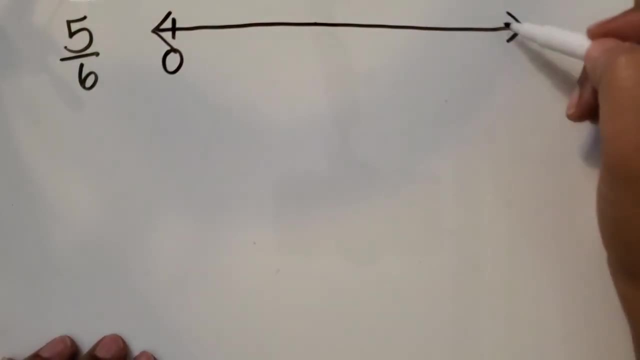 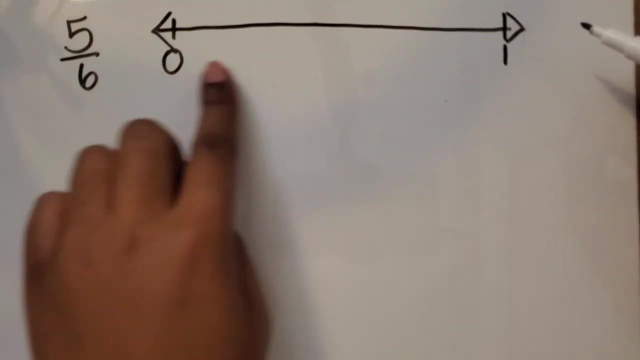 If I wanted to represent five, six, I would draw my number line to represent a hole And looking at my fraction, I see that six is the denominator. So I know I need to break or partition, Break up or partition the hole into six equal parts. 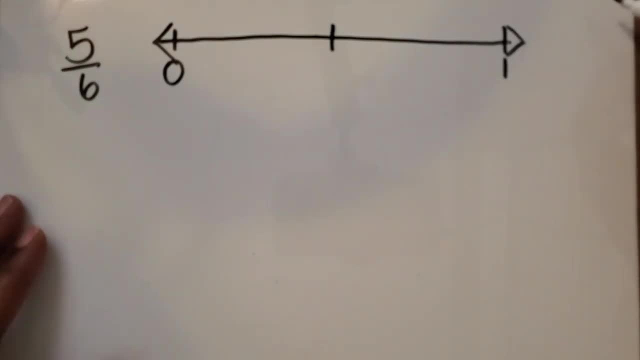 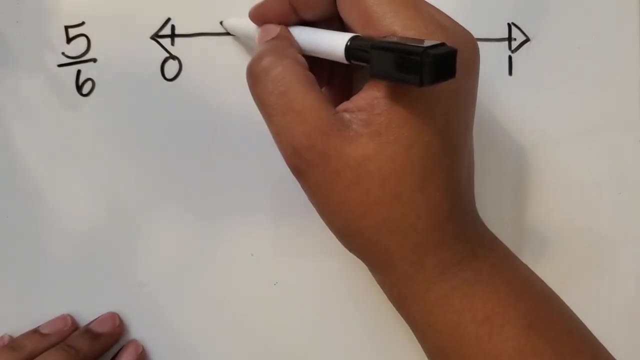 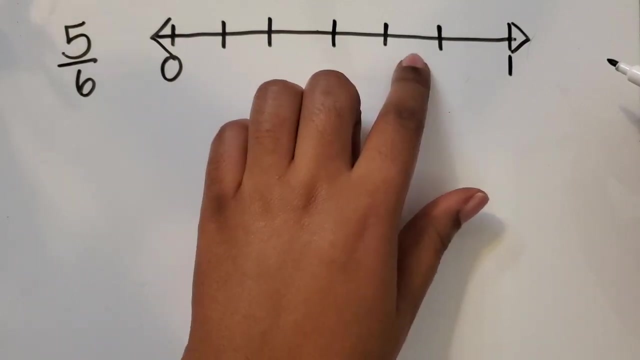 So I'm going to start by partitioning it in half, first because it's an even number, And then for each half I need three on this side and three on this side, Three spaces. So I'm going to partition each half into thirds, for a total of six equal parts. 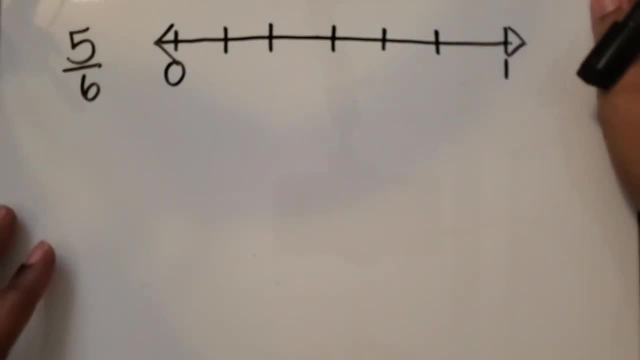 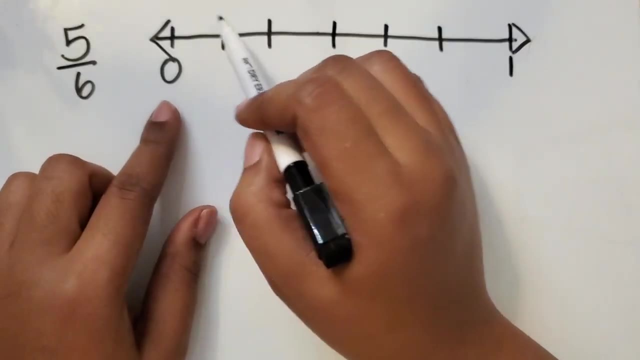 So where is five, six on the number line. So if we're at zero, from zero to one hole, We know there's six equal parts. So from zero to the first tick mark is going to be one six. The second mark is going to be two six. 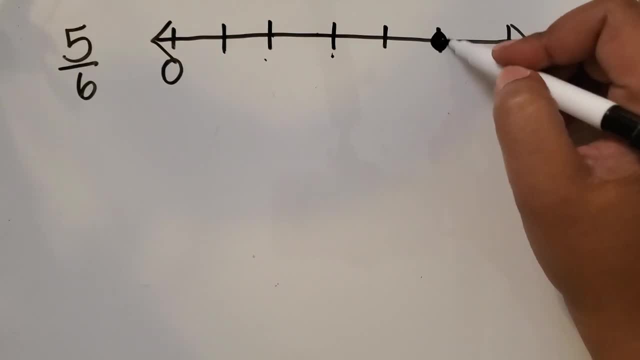 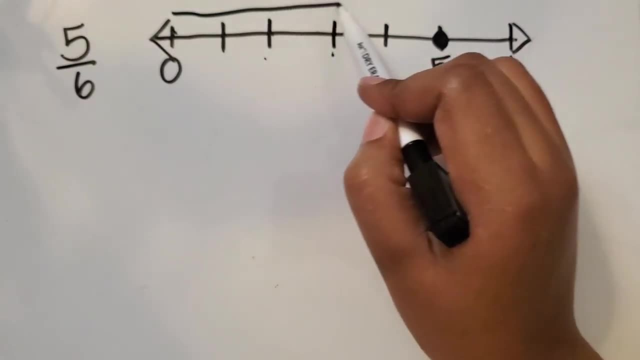 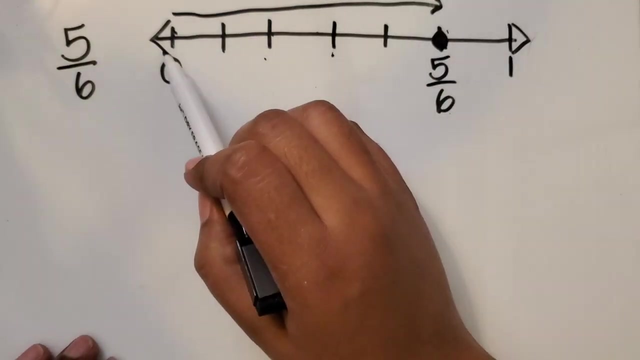 Three, six, Four, six. Here is where five six will be on the number line. So from zero all the way here it represents five six. Not just this point, but from zero to this point is a length of five six.